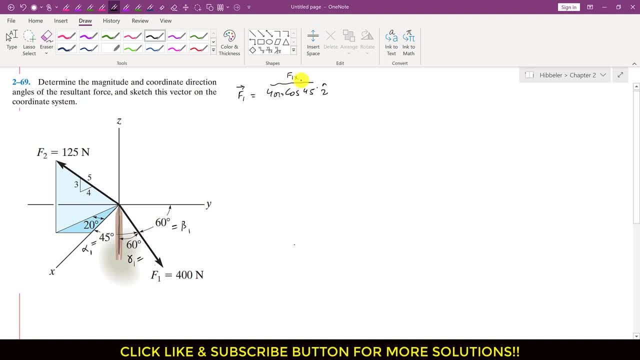 Y right. this is f1 X right. similarly I will write f1 Y. so we can write: f1 Y is 400, cause of 60 degrees, right J. and similarly we can write: this will be f1 Z component right. so f1 Z in terms of: 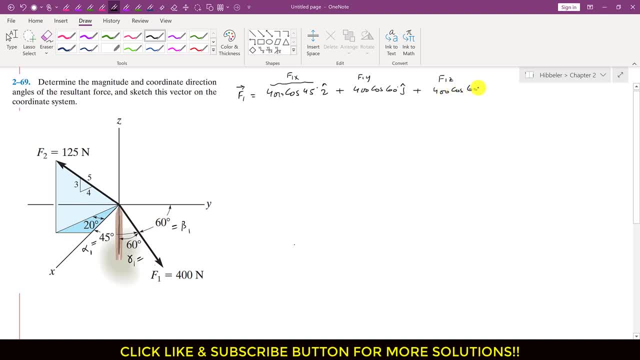 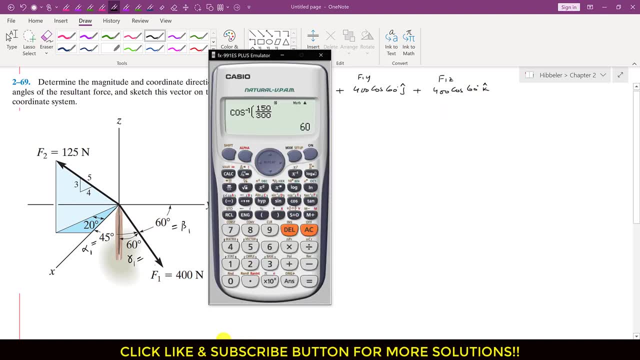 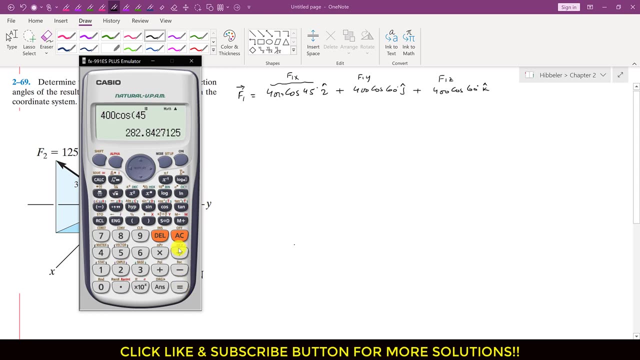 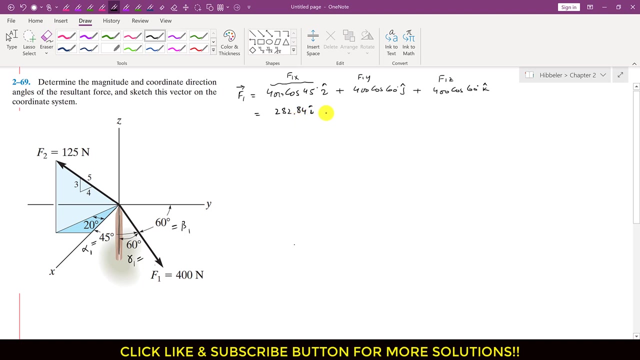 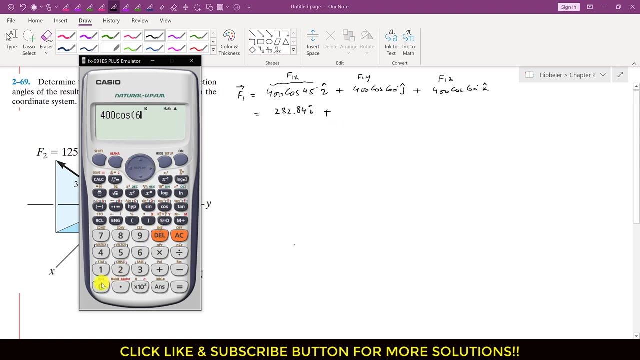 gamma 1 will be 400 cause of 60 degrees. right, and this is in the K direction. so this is f1 vector. we can simplify it right. so f1 is 400 cause of 45, this is 282.84. I plus this 400 cause of 60, this is 200. J plus 400 cause of 60 is, again, it is 200. 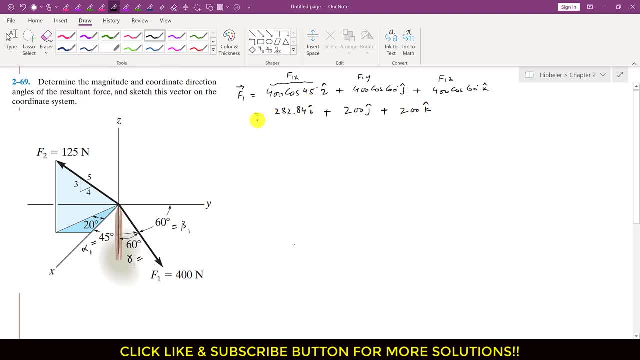 right, so we can write: it is 200 K, right. so this is f1 vector, Cartesian vector, right. similarly we can write f2, right. so first the this angle is given in terms of this triangle. so if we are considering this angle, let's say that this angle is theta. so 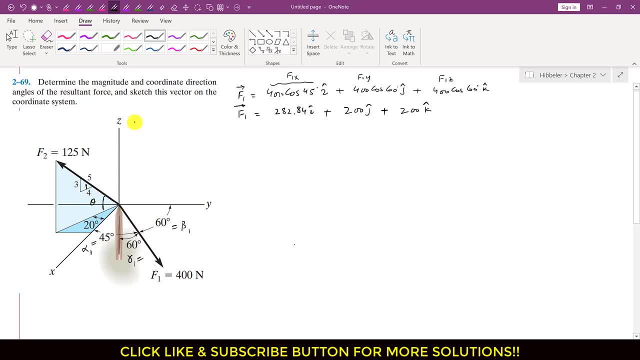 then from this triangle we can find this theta. so if I apply 10 theta to this triangle, so 10 theta, so this triangle will be perpendicular divided by base right. so this will be 3 divided by 4, so we can find theta. it will be 10 inverse 3 divided by 4. 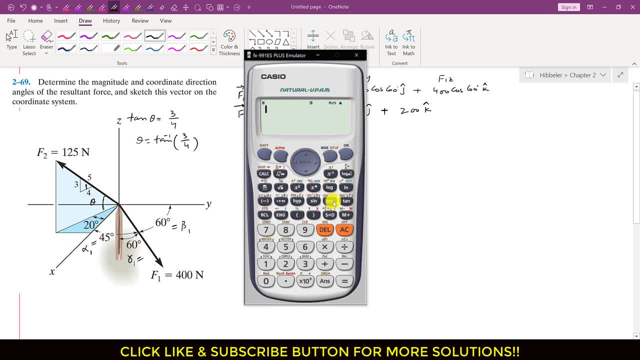 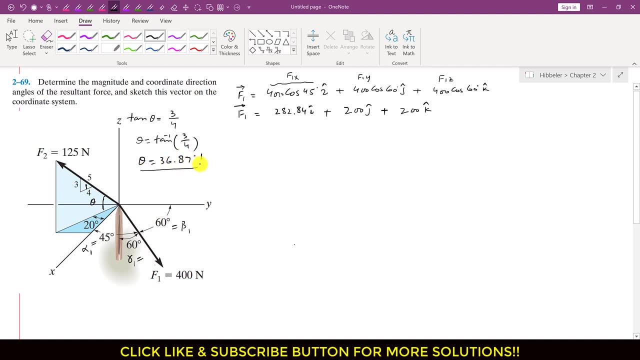 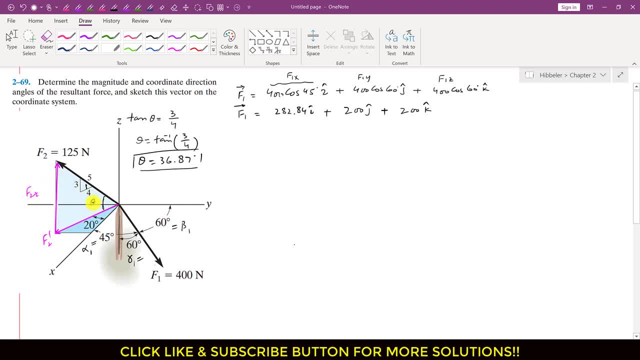 z component. this is a 2 z component right. so if we consider this light blue triangle, then f2 dash. i can write that f2 dash is the cost component. we can write that this is 125 cos of theta right. 125 is that 2 magnitude and theta is 36.87. 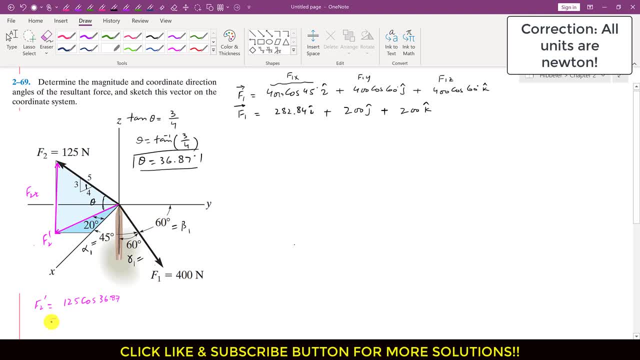 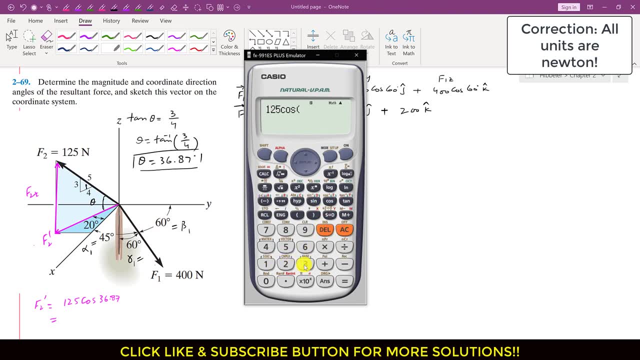 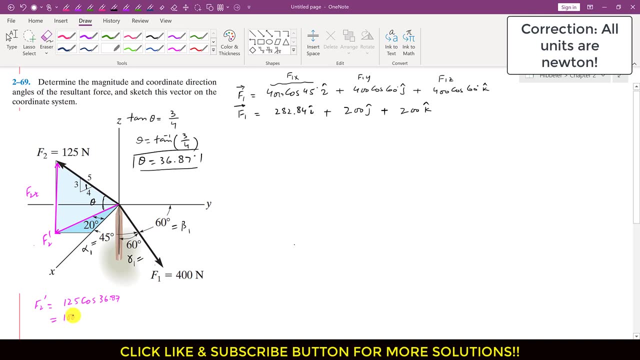 all right, so we can find f2 dash. so f2 dash is a 125 cos of 36.87. so this is 99.99. so we can write that this is 100, right, this is 100 pounds. similarly, uh, this f2 z will be the sign component, so i can write that f2 z is 125. 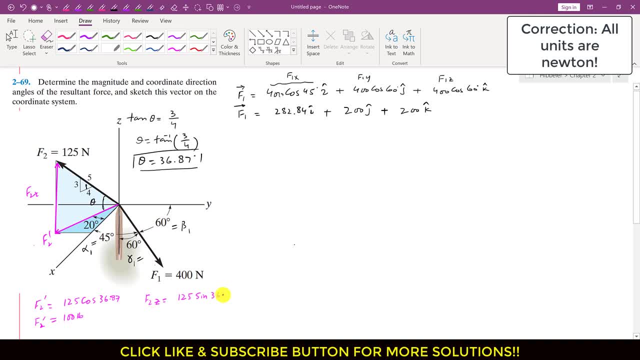 sine of 36.87, right? so this will give us 75 pounds, right? so f2 z is 75 pounds, and if two z is acting in the positive direction, f2 dash is 100 pounds. so now, if i resolve, uh, this have two departed further. 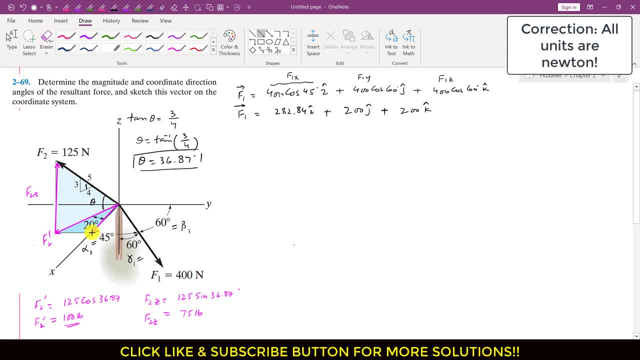 into two components. right, so this is two dash. we'll have one component like this: so this component is acting in the positive x direction. so we will bebag hi this: so this component is acting in the positive x direction, so we can write that this is f 2- x and similarly, it will have one common which will be acting in the 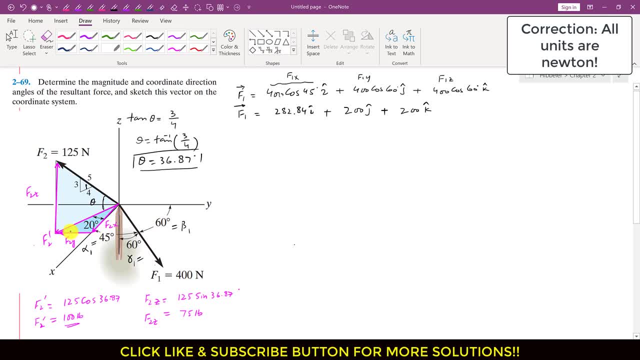 negative y direction. right, so this is f 2 y. right, so we can write f 2 vector, so f 2 vector is equal to. so now we can write that f 2 x, right, so this is f 2 x and this is the cos component of f 2 dash. 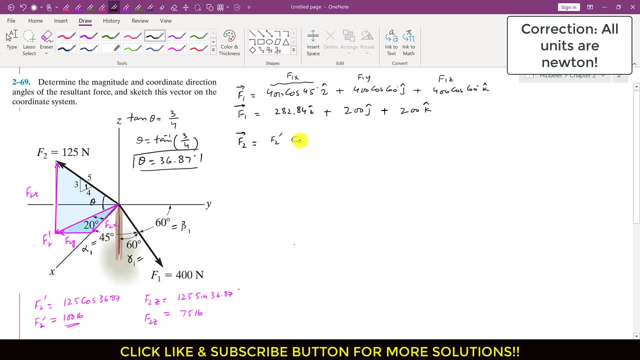 right, so i can write that f 2 dash cos of 20 degrees right. and this is acting in the positive x direction, so i will write positive i. and similarly, f 2 y is acting in the negative y direction, so i will write minus. and this is the sine component of f 2 dash right, so i can write: 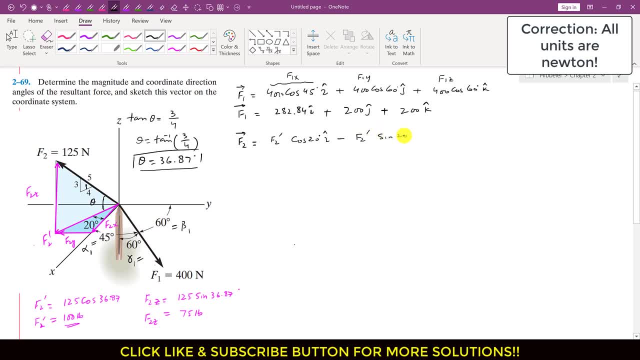 that f 2 dash sine of 20 degrees, right, and this is acting in the positive, negative j direction, so this is negative j. and similarly f2 z is acting in the positive z direction, so i'll write plus, and this is the f2 z is 75 pounds, right, we have determined this right. so this is 75 positive t. 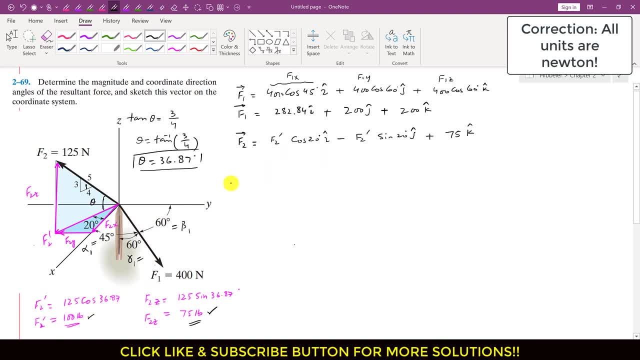 so now, as we know that f2 dash is 100 pounds right from here, so we can write that up to- we can replace f2 dash with 100, right? so this is 100 cos of 20 and this is 100 sine of 20.. 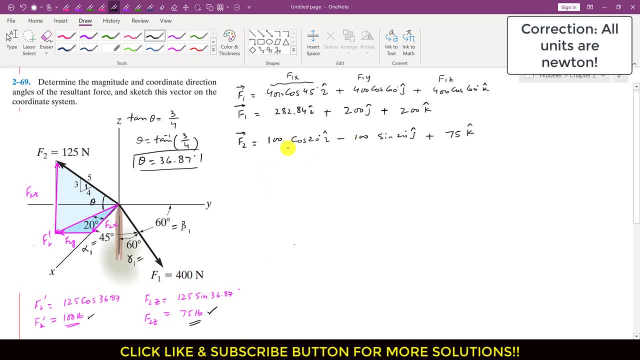 we can simplify this, right. so before simplifying this, let me add f1 and f2. right? so the summation of f1 and f2 will give us the resultant cartesian vector. right, so the resultant cartesian vector. so if we add the corresponding f1, x and f2 x component, so that will give us the rx component. 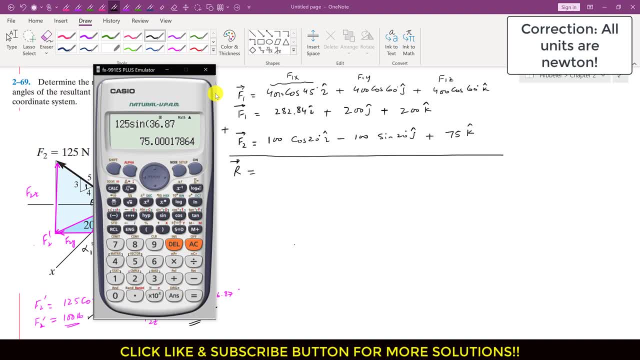 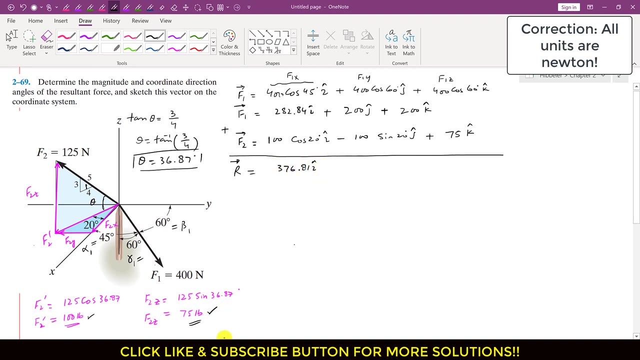 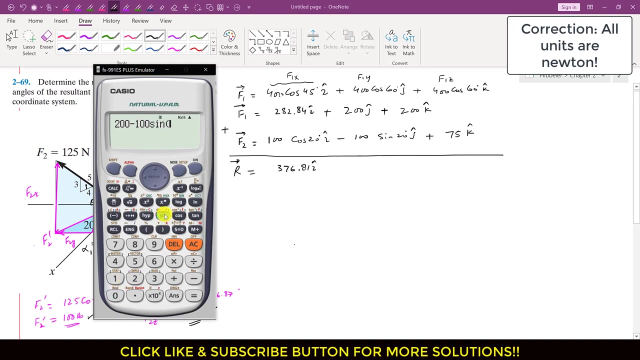 right. so if i add this 282.84 and this component- right so- this is 282.84 plus 100 cos of 20.. so this is equal to 376.81, so 376.81. i similarly 200, 200 minus 100 sine of 20.. 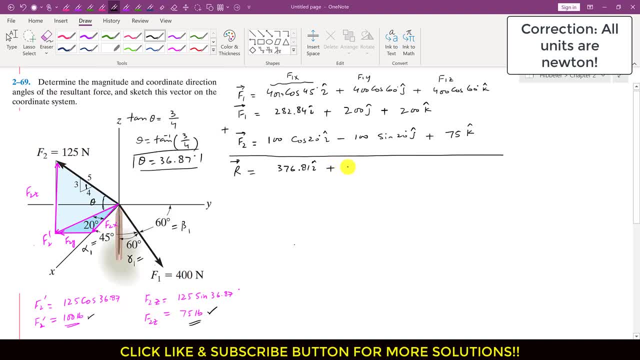 this is 165.80. i write minus 165.80. now if we add, uh, the f1 z component and f2 z components, so that will give us the resultant rz component, right? so but here is, we can see that this f1 is acting in the downward direction, right. 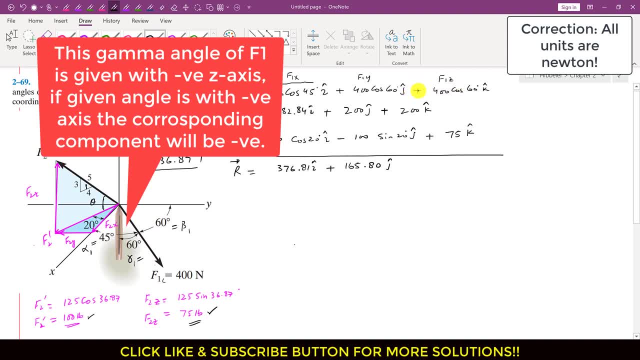 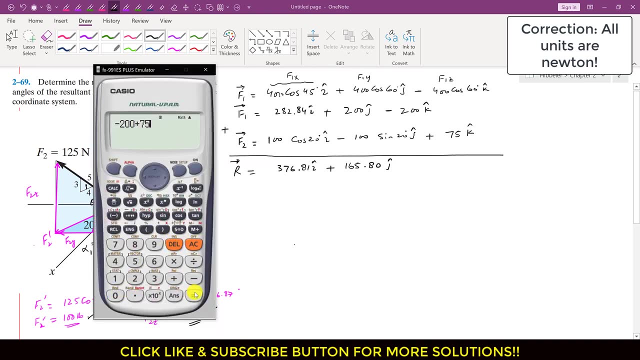 so f1 z is negative, right, so here i have written it positive. but this is negative, right, so we will write that this is negative. so if this is negative, then this is minus 200, right? so minus 200 plus 75.. so this will give us the r z component. so minus 200 plus 75, so this is minus 125, right? so i will. 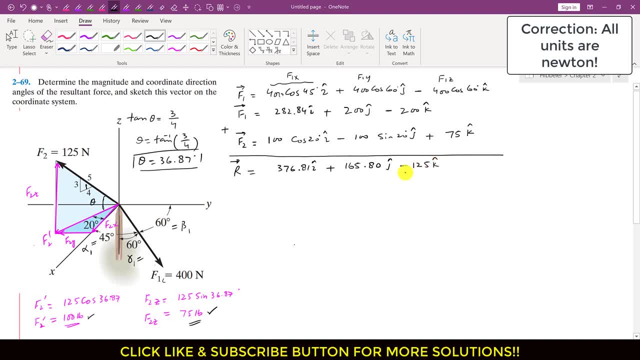 write minus 125, key right, and to find the resultant magnitude. it is said that find the resultant magnitude so we can find: this is rx, this is r1, this is rz. so the resultant magnitude will be equal to 376.81 squared plus 165.80 zero square plus 125 squared, and then we will take the square. 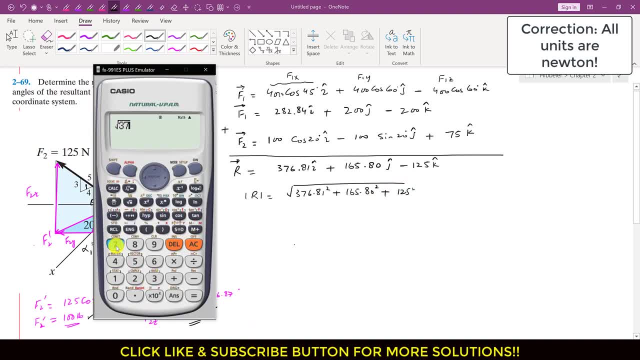 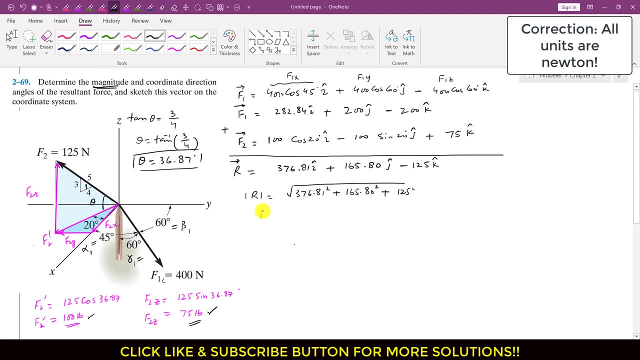 root. so this is, uh, 376.81 squared plus 165.80 squared plus 125 squared, so the resultant magnitude is, let's say, approximately 430, right? so i will write that this is approximately 430 pounds, right. and to find the coordinate direction angles, as we know that, 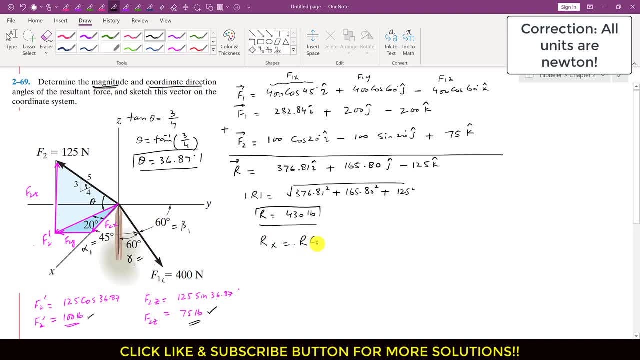 rx is equal to r cause of, let's say, alpha. let's say the resultant is making alpha angle with the positive x axis right. so r cause of alpha will be equal to 376.81, right. as we know, this is rx. so from this we can write, we can find. 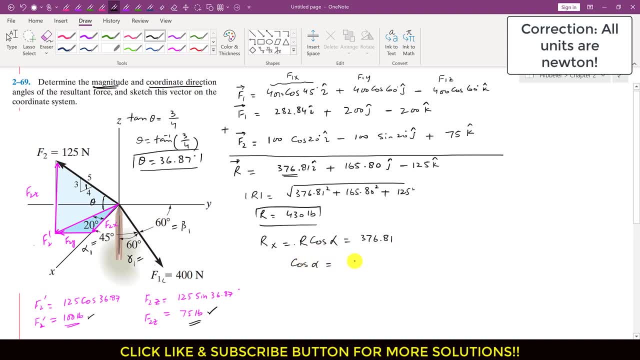 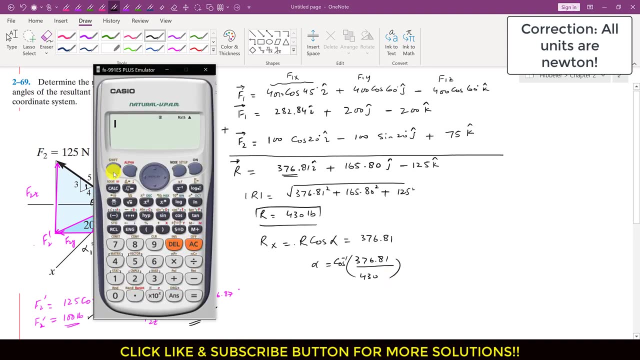 alpha. so cos alpha is equal to 376.81 divided by 4, 30. and if i take cos inverse, so that will give us the angle of the resultant with the positive x axis is right. so cos inverse, we can write that cos inverse 376.81 divided by 4, 30. so this is 28.79, right? so i can write that this alpha. 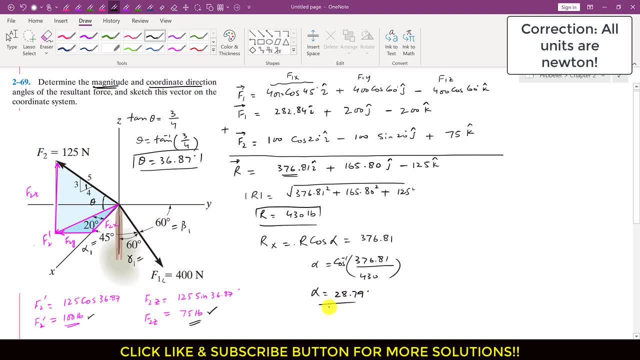 angle is 28.79 degrees. similarly, we can write that r? y, in terms of the coordinate direction angle, will be equal to r cos of beta. beta is the angle of the resultant with the positive y axis, so this will be equal to 165.80. so from this we can write: beta equals to cos inverse 165.80 and divided by the resultant. 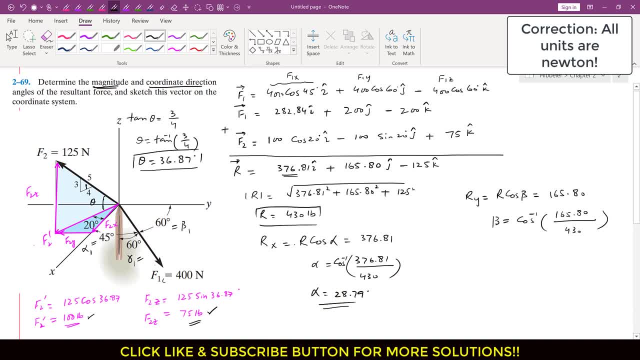 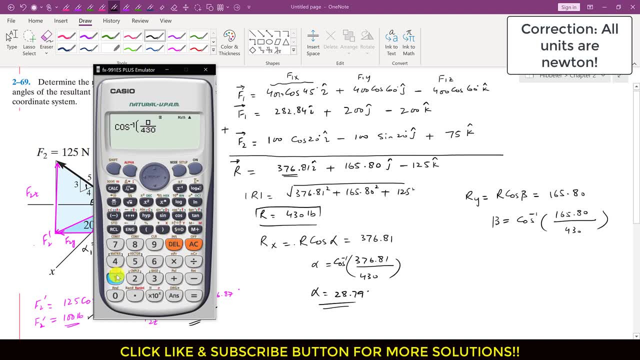 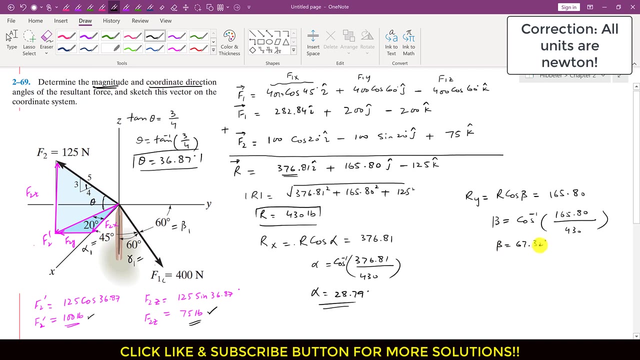 in magnet orbit is 430. this is one sixty five point eight, zero. so from this equation, beta is sixty seven point three, two. beta is sixty seven point three, two degrees. and similarly we can write that our Z in terms of the direction coordinate, direction, angle, this is equal to our cause of gamma, so from which is: 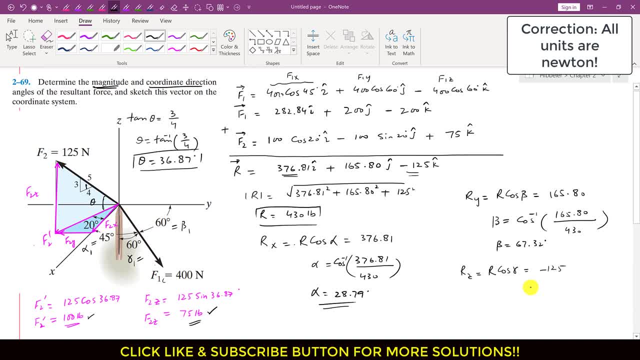 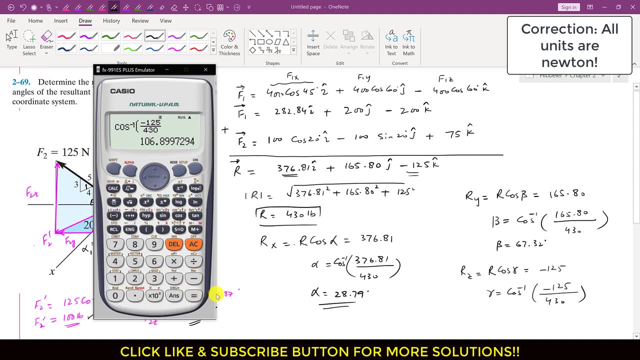 equal to minus 125. so I will write: it is minus 125 and from this gamma will be equal to cos inverse minus 125 divided by 430 minus 125. so this is hundred and six point eight nine. so we can add that this is hundred and seven approximately. right, this is hundred. 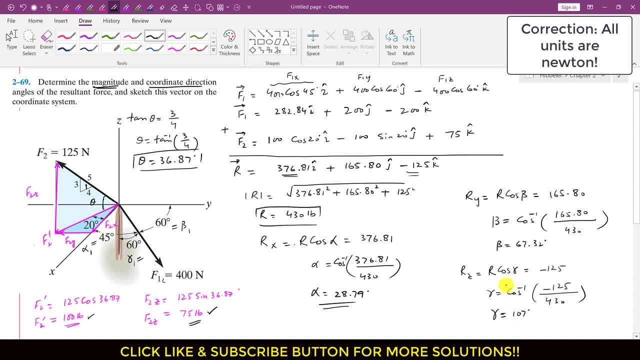 and seven degrees. so in the problem it is said that also sketch that resultant vector, right, so let me sketch it. so let's say that this is my positive X, positive Y, and, sorry, this is my positive X, this is my positive Y and this is my positive Z. axis is right. so now is we can see that the resultant has one. 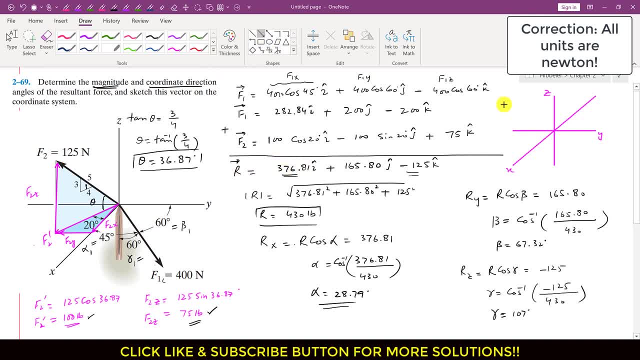 component is acting in the positive X direction, right? so let's say that this is our X. let's say: and it has one camera which is acting in the positive Y direction. so let's say: this is our Y and it is one. it has one camera which is acting in the negative Z direction, right? 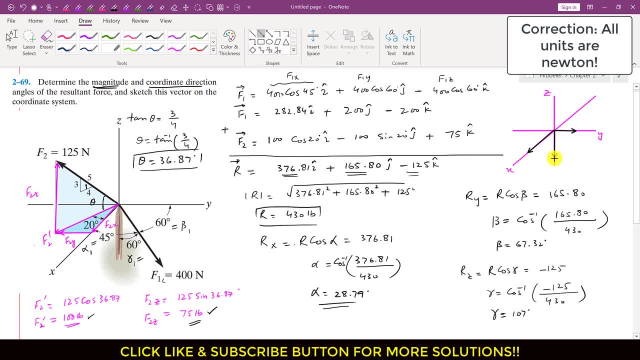 so let's say that this is our Z right, so we need to add these three components in order to get that resultant right. so if I place this, our Y component, here and if i place this rz component here, right, so this is the resultant vector, right. so, from the tail of rx. 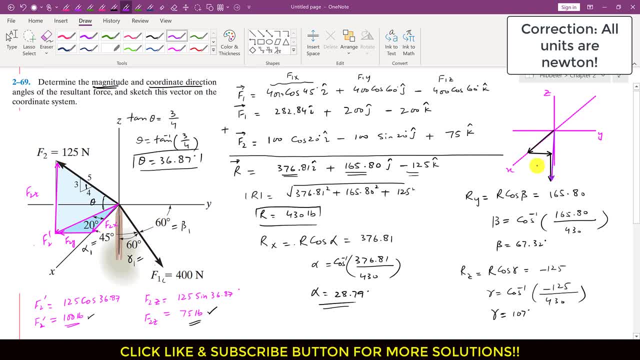 to the head of rz. right so, if i erase these components now, right so, this is the resultant vector. right, so now we can say that this resultant vector is making alpha angle, this alpha angle with the positive x-axis, whose magnitude is 28.79. it is making beta angle with the y-axis, like this: